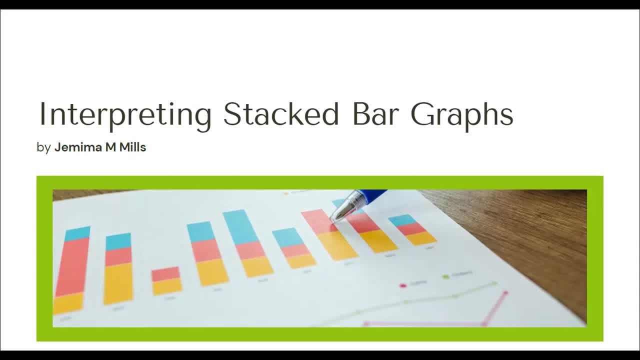 This one. it's a bit more complicated and normally students get in kind of a They have kind of an issue in understanding or what I should say, interpreting these bar graphs. So let's get into it and let's know how we should go about answering these questions that they may pose on the exam surrounding stacked bar graphs. 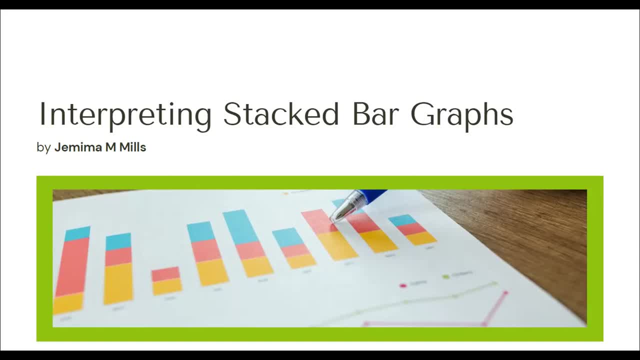 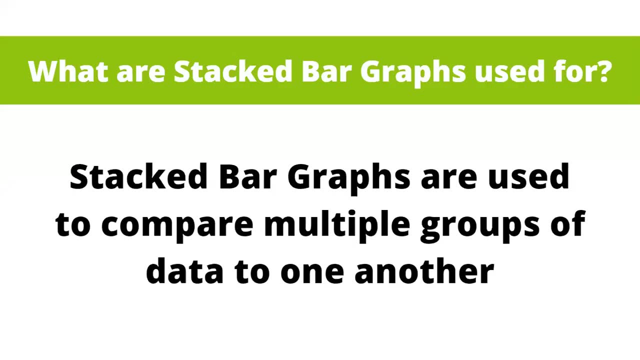 So the first thing we need to know is: why are stacked bar graphs used? So, stacked bar graphs are used to compare multiple groups of data. So, for example, in the environmental science exam, they may give you some crops and they may tell you that in this year this is the amount of crops that will produce, and they would give you the unit, whether it's in tons, whether it's in kilograms, and they would ask you some questions. 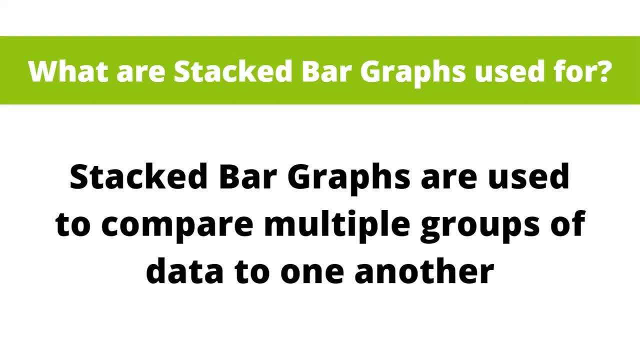 Like they would put this on the stacked bar graph and they'd ask you how many tons of this crop was produced in that year, or how many tons of that specific crop. No, not that I said that already. Like for that year, how many tons were produced for all the crops? 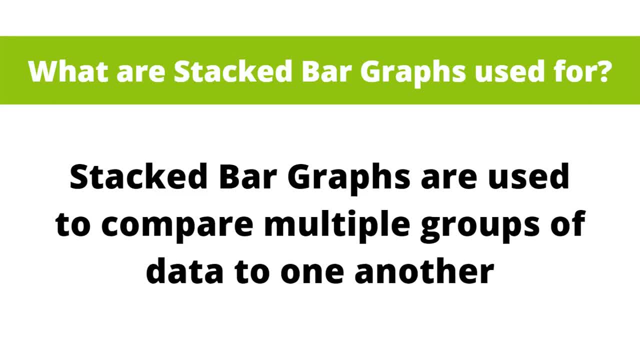 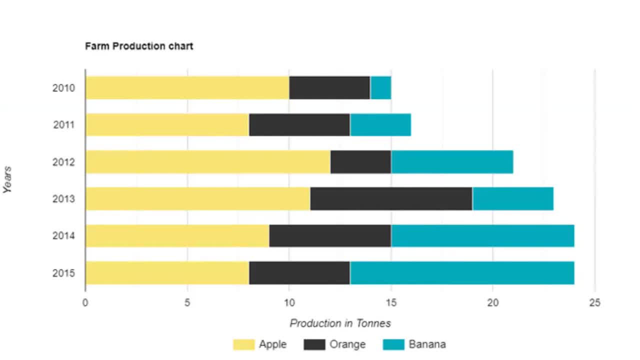 Yeah, that's the better way to phrase it. So, yeah, And the one I actually have. it's like the exact question. This one is a farm production chart and it's a stacked bar graph, of course, and it shows the production in tons and years. 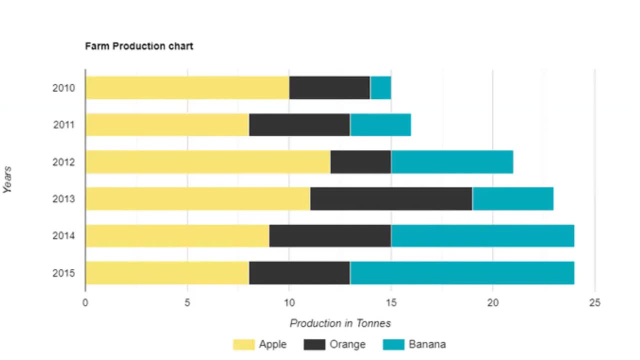 So the years we have is 2010,, 2011,, 2012,, 2013,, 2014, and 2015.. Now this video is going to be really short, because it's just a really short explanation and straight to the point. 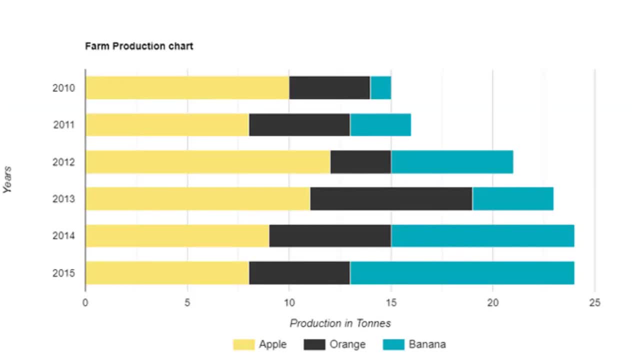 So we don't want to keep the video more than 10 minutes per se. So I just want to go straight to the point and ensure that you guys understand it, And if you don't, just comment below and tell me that you don't understand, and I will be very willing to explain it to you guys. 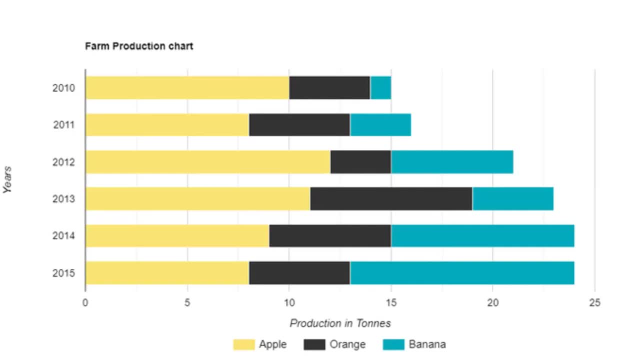 Also, if you hear any background noise, that's my dog, so I apologize in advance. So let's see. They ask us: We have apples, we have oranges and we have bananas. So they ask us: what was the production in tons for apples in 2010?? 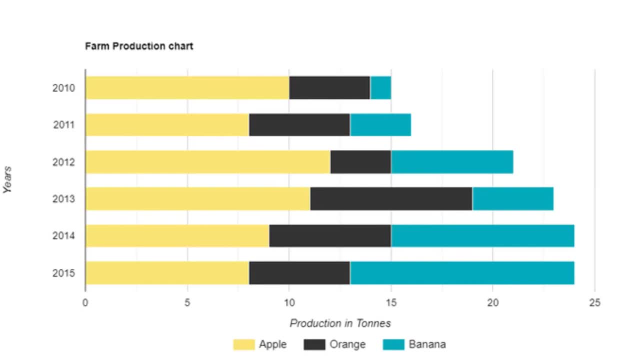 So we go to the x-axis, We see 10. So we know that is 10 tons. But what if they ask us what was the production in tons for oranges in 2010?? So if you don't know, for example, if a student doesn't know how to interpret the stacked bar graphs, 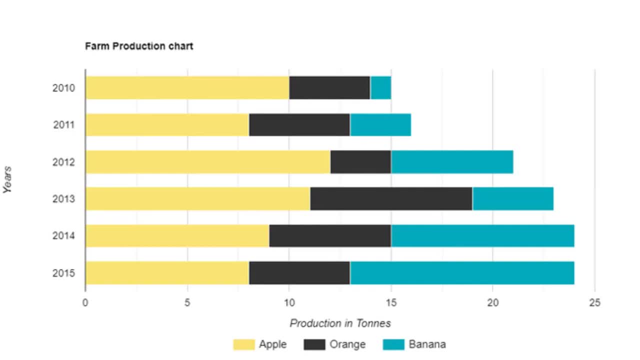 they may just say. they will say, let's say you know apples is 10.. Then you know, the middle value looks like 12.. And this, where the value for oranges is, it kind of looks like 14.. 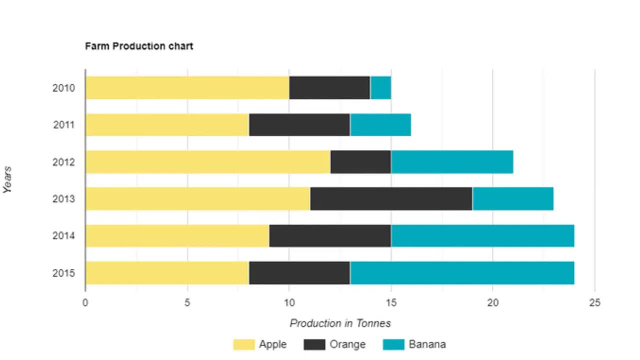 So you would say 14 tons of oranges. No, that's completely wrong For stacked bar graphs. it's a bit more complicated And it's not extremely complicated. It's just simple mathematics that you have to use. So for you to find the value of the oranges, you would have to say the 14 minus the 10.. 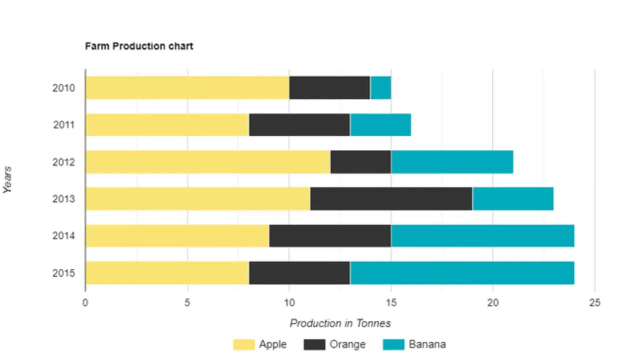 And that would give you 4 tons. If you want to find the value of the bananas, it would be, so it reaches 15.. You'd say 15 minus the 1 before, or not even the 1 before, actually the 1s before. 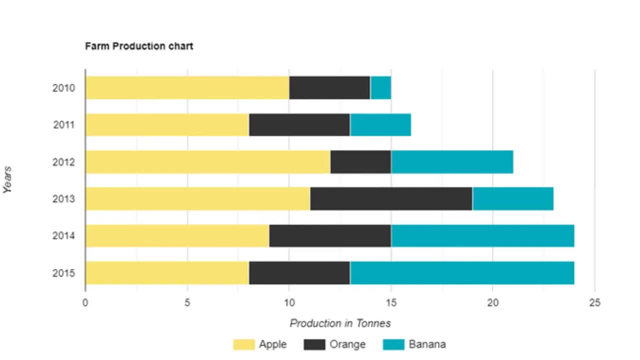 So remember you had 10.. Then you had 4.. So you would say 15 minus 10 plus 4. That is 14.. And that will give you only 1 ton, And this is how you would do the rest. 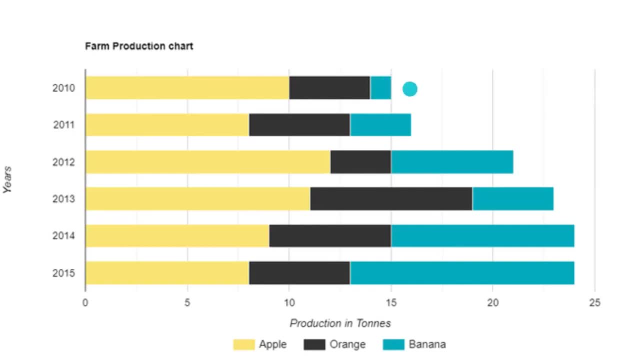 So the example. so let's say, if there was one right after this, you would have to subtract the value for wherever it reaches, minus this one, this one and this one, And for all of your stacked bar graphs. this is how you do it. 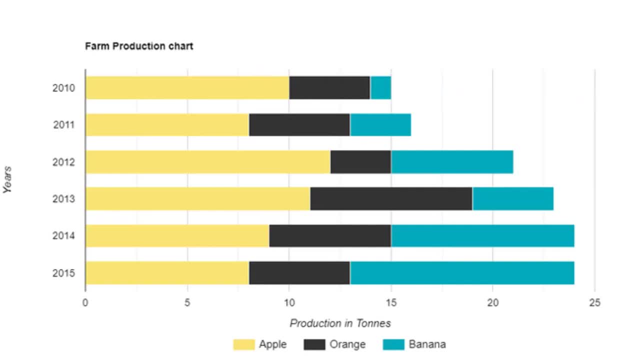 It's just as simple as that. So I really hope you guys understood this And, if you don't, as I said before, just comment, And if you do, share this with your friends. So if, in case, they have any issues understanding stacked bar graphs, this can really help them understand it. 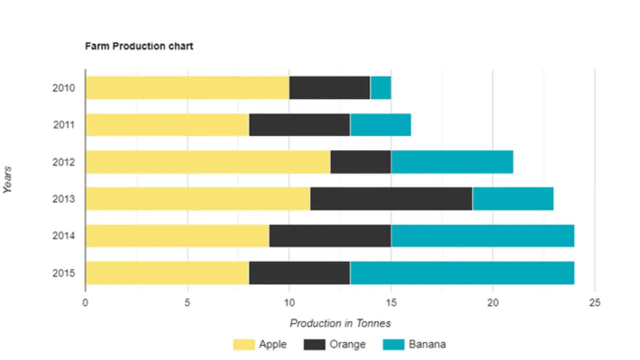 So remember, it's just simple mathematics. You minus the 1 that you're doing to the 1 you did before or the 1s you did before, and you get it To get the. let's say you want to find the complete value for 2010,. you would add all of them together.